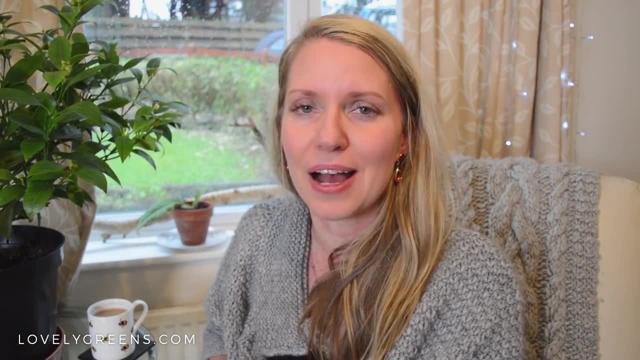 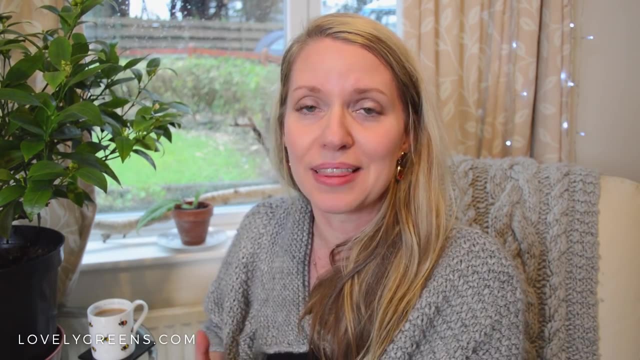 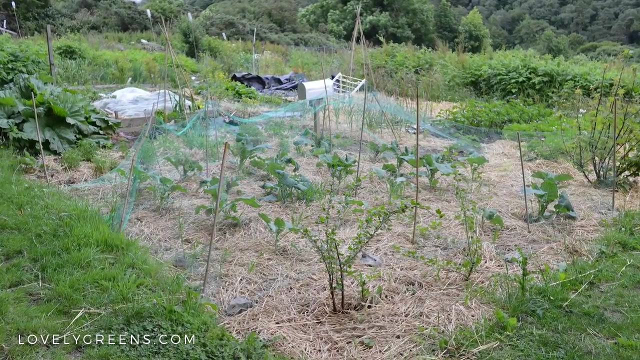 and just letting time and the UV consistent black plastic just do the work for me. it saved a lot of time. So I started off my plot by doing that first. And then I cultivated a bit, grew a few things, I experimented with some straw mulch. 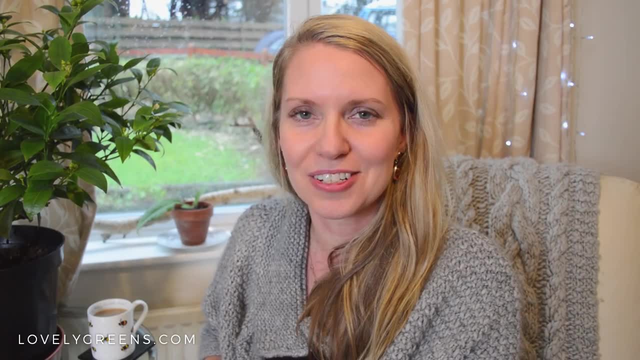 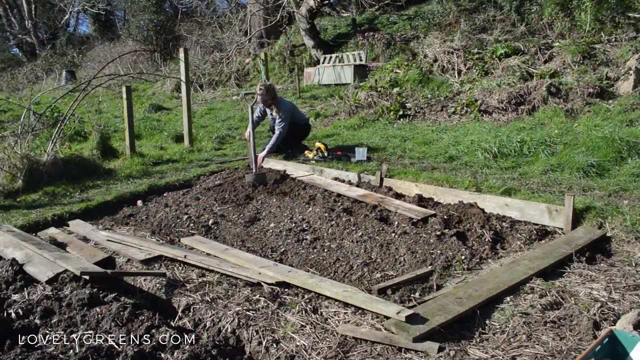 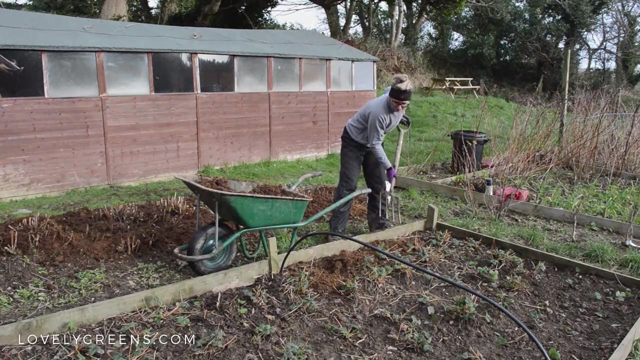 which was a terrible idea. There were so many slugs. But then I moved on this last year with creating raised beds, using composted manure as a mulch and as a soilestoist supplement and also creating paths, so that has saved so much time and effort. 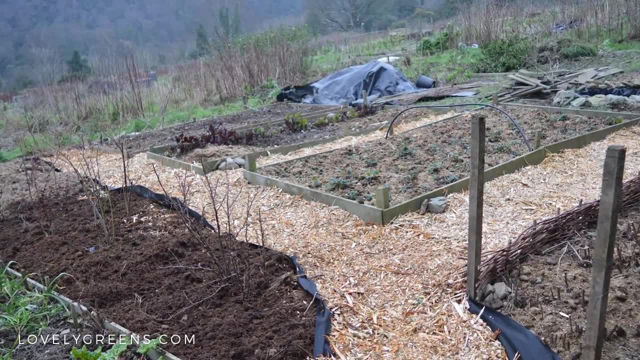 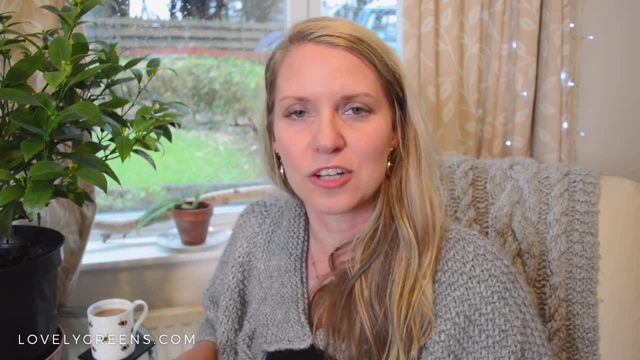 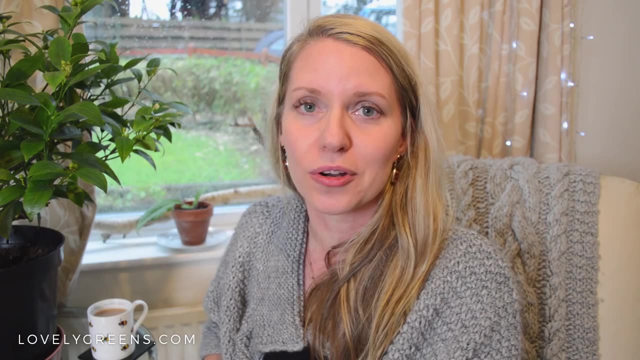 as well in actually maintaining my plot, because you know, it's one thing to keep your beds weeded and your vegetables weeded and to focus your attention on that, but when you're also dealing with overgrown pathways that you have to strim or weed, then it's even more work. so last February I actually put down 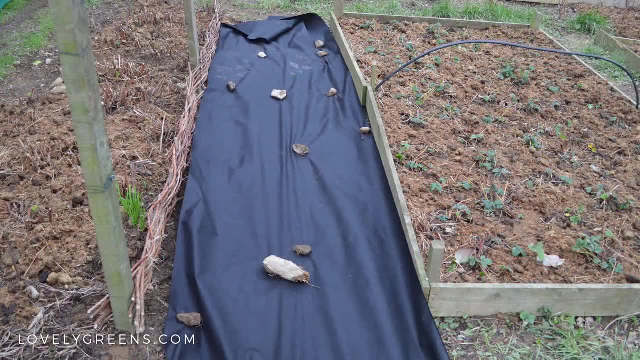 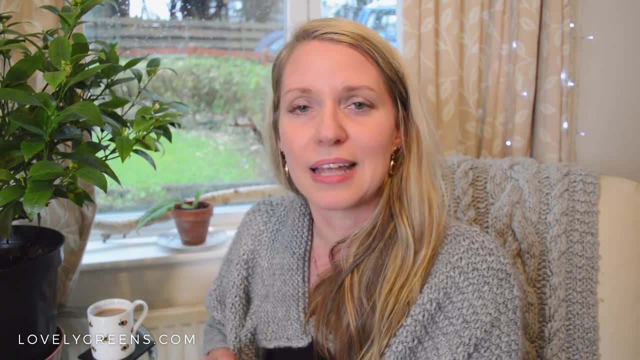 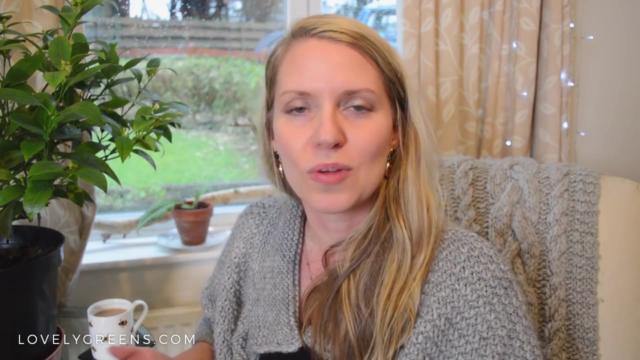 some horticultural material on the ground and then covered it with wood chips that we got for free at the allotment, and it has been probably the best idea for creating a plot that I've actually used, because even when I've been away on holiday- so last last summer I was in Portugal for a month- came back. 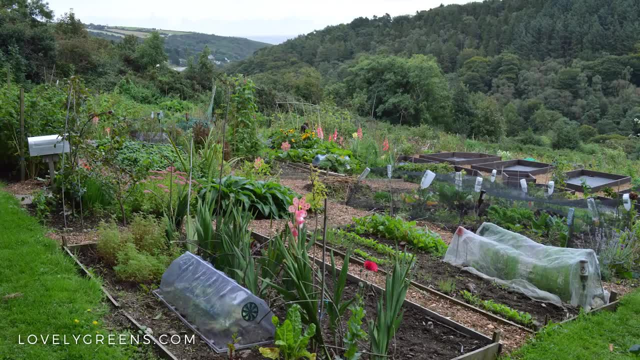 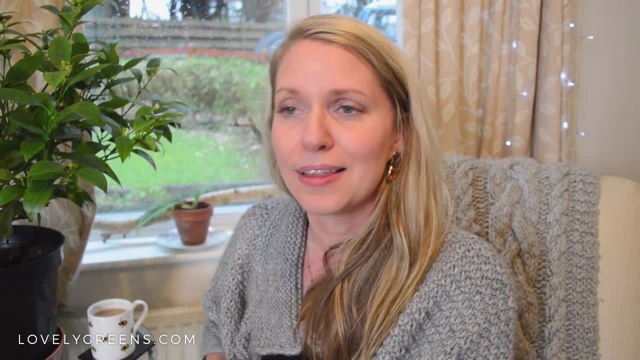 and the paths were virtually cleared, whereas in the past, if I would have been away for even a couple of weeks, I would have gotten back and it would have just been a nightmare. so I would highly recommend putting in wood chip paths. and the other thing is is that you can often get wood chips for free. so if 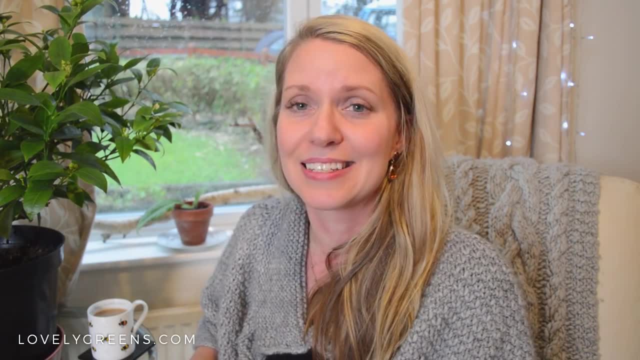 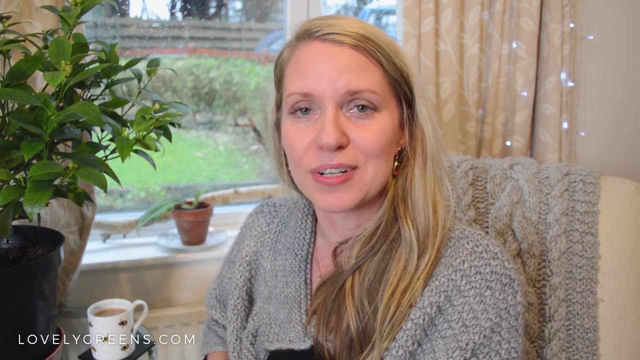 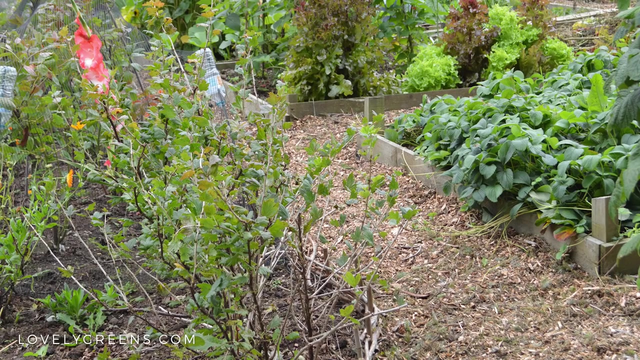 you've got a tree surgeon in the area, they'll often either sell it very inexpensively or give it free because it's just a waste material for them. and in fact we have a very generous tree surgeon in Laxey who just regularly just dumps off wood chips for us because we use them for our paths, etc. another thing: 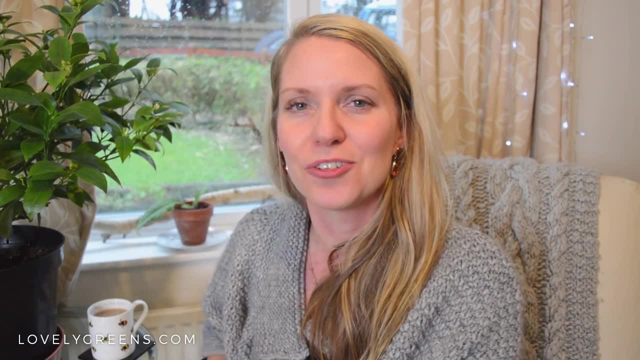 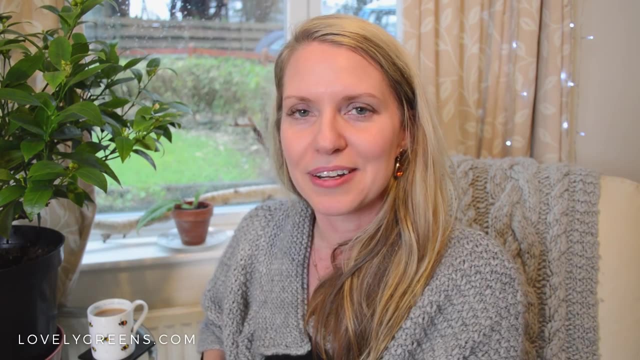 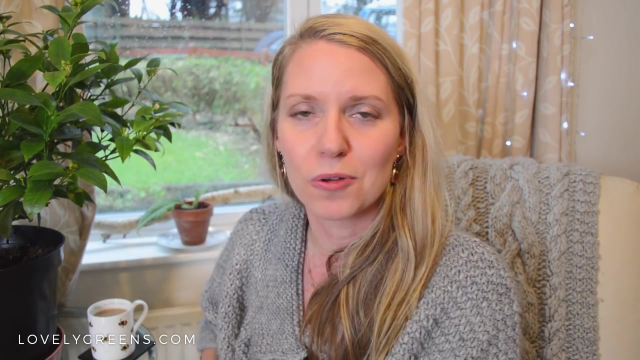 that I started doing last year, in which I will continue to do this year, now that I have more material- is you prune your raspberries, your autumn fruiting raspberries in the winter time, and normally what happens to the canes is either burned or composted, or I've gotten gotten rid of in some way and I 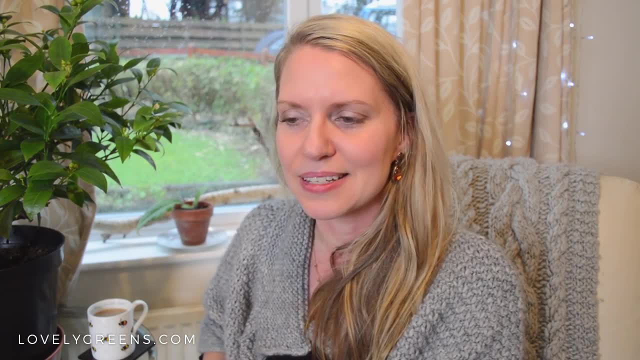 was looking at these canes for a while and I had them in a stack and then I I decided I'm gonna try using them as a material in the garden. and so I decided I'm going to try using them as a material in the garden and 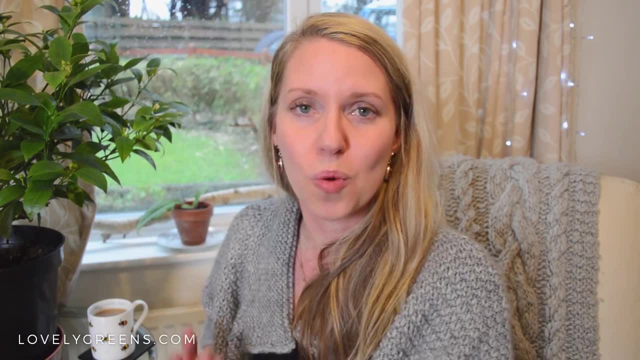 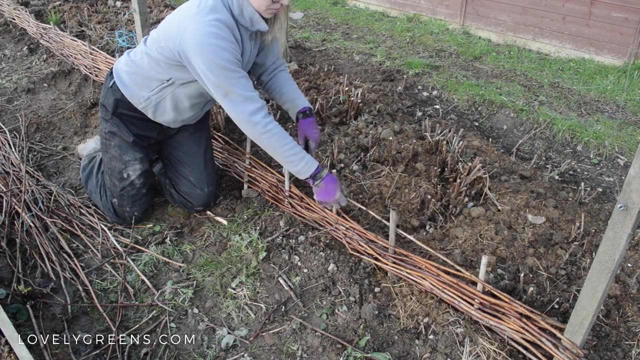 and so I decided I'm going to try using them as a material in the garden, and last February I started putting in some wattle edging in the allotment and it looks so pretty and I don't think that I'd seen it before. I mean, I'd seen it. 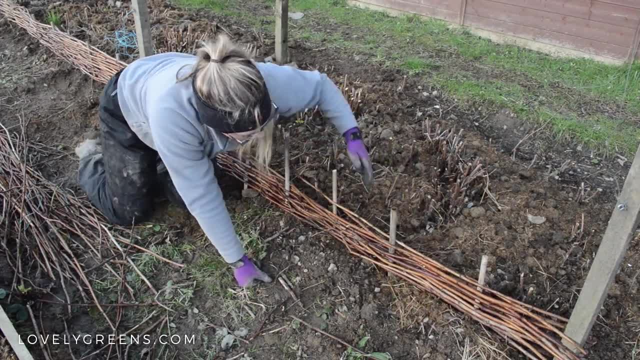 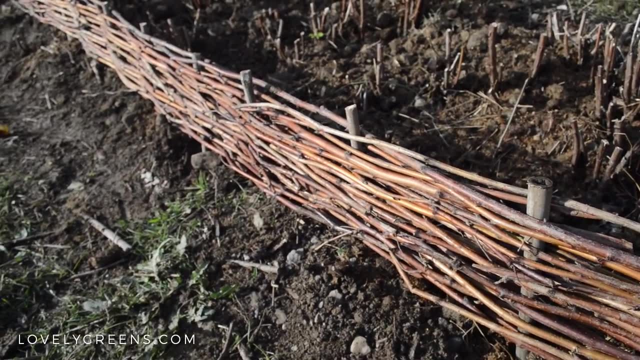 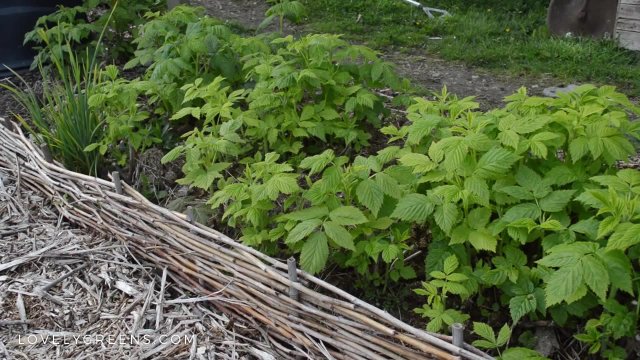 wattle edging and wattle features made with willow and hazel but never with raspberry prunings, and it actually has held up as well. I think a lot of people might think, hmm, you know, after a season or so, you know it probably wouldn't have. 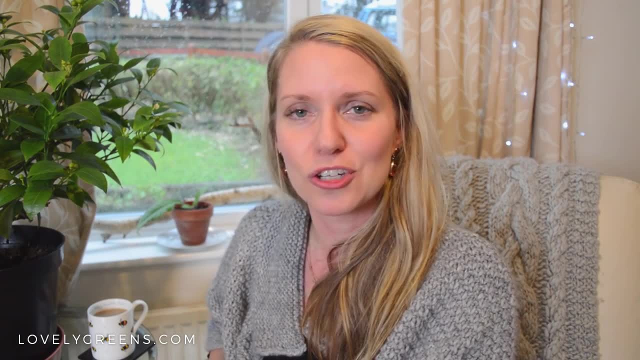 that longevity, but it looks really great that longevity, but it looks really great and I will continue edging my beds and I will continue edging my beds in that. so if you are pruning raspberries in that, so if you are pruning raspberries about now, which a lot of people will be, 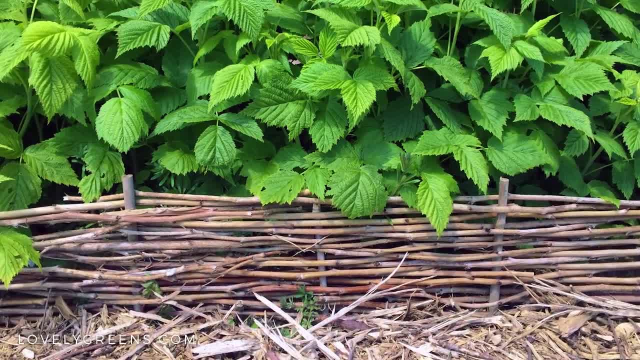 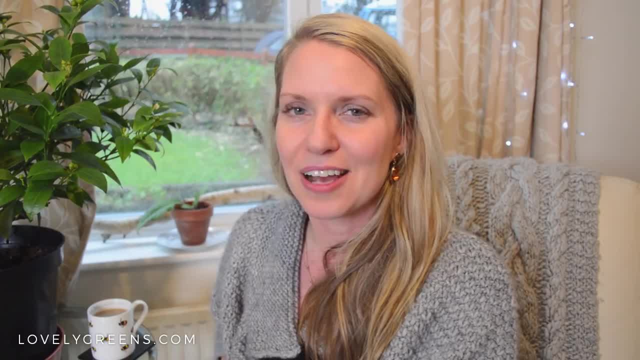 about now which a lot of people will be doing: keep those prunings and create some doing. keep those prunings and create some. some garden edging with that. another, some garden edging with that. another thing that I put into my allotments, thing that I put into my allotments around this time last year, was a small. 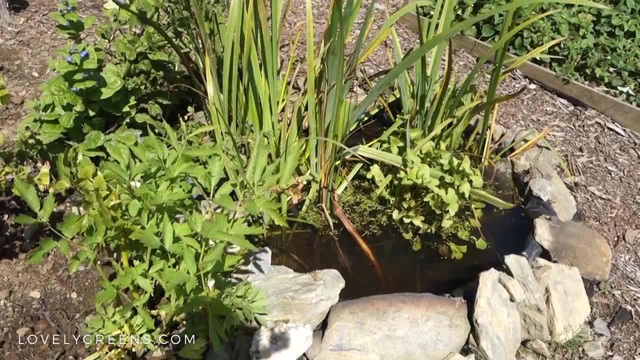 around this time last year was a small pond and actually the kind of a- the tail pond and actually the kind of a. the tail end of winter is an ideal time to put in end of winter is an ideal time to put in a water feature like a pond, because you 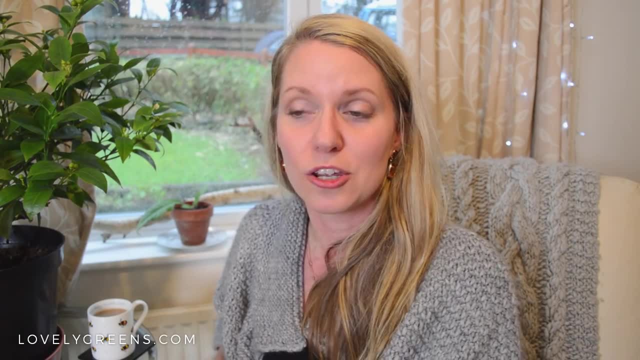 a water feature like a pond. because you a water feature like a pond, because you are preparing it for spring. you, you know, are preparing it for spring. you, you know, are preparing it for spring. you, you know you don't have very much to do in the. you don't have very much to do in the. 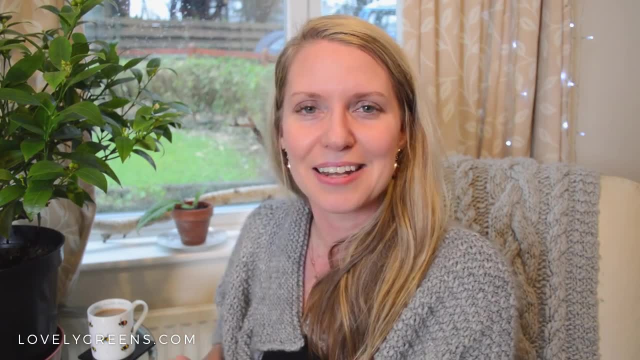 you don't have very much to do in the allotment or in the garden at this time allotment or in the garden at this time allotment or in the garden at this time of the year, so you can dedicate it to. of the year, so you can dedicate it to. 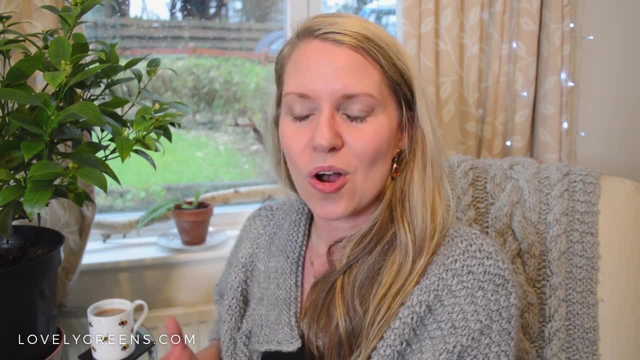 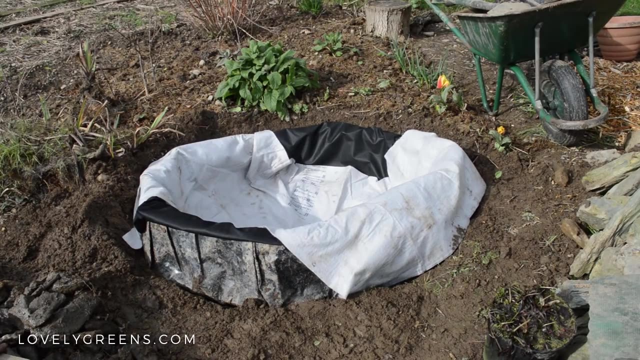 of the year so you can dedicate it to putting in features like that and all it. putting in features like that and all it. putting in features like that and all it involved was digging out a hole I lined. involved was digging out a hole I lined. involved was digging out a hole. I lined it. so I put down some fleece first and 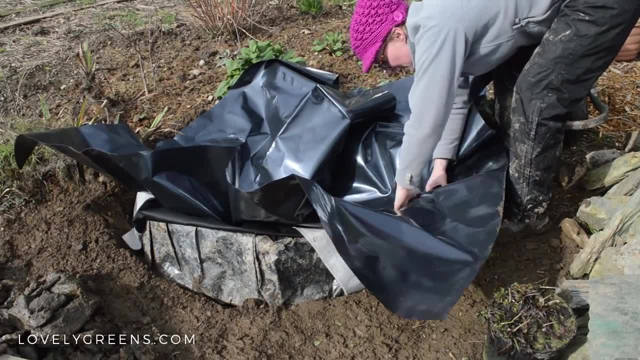 it. so I put down some fleece first and it. so I put down some fleece first and then the actual pond lining, and then then the actual pond lining and then then the actual pond lining, and then weighed it down a little bit filled it, weighed it down, a little bit filled it. 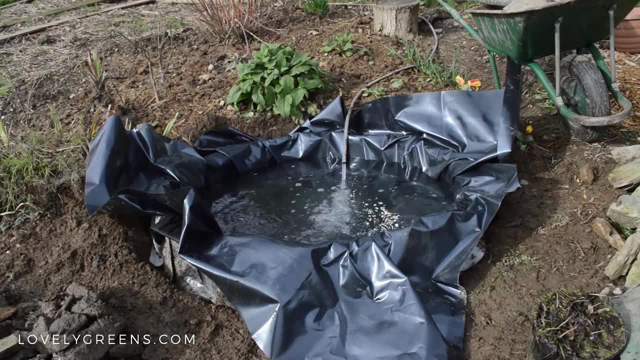 weighed it down a little bit, filled it with water, edged it with rocks and it with water, edged it with rocks and it with water, edged it with rocks, and it has attracted so much wildlife to my, has attracted so much wildlife to my, has attracted so much wildlife to my garden this year, or last year rather, 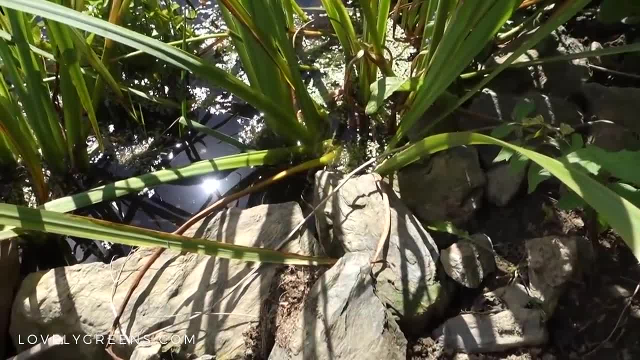 garden this year or last year, rather, garden this year or last year, rather, which is fantastic, because that was the which is fantastic, because that was the which is fantastic, because that was the intention, as well as to create a haven, a intention as well as to create a haven, a. 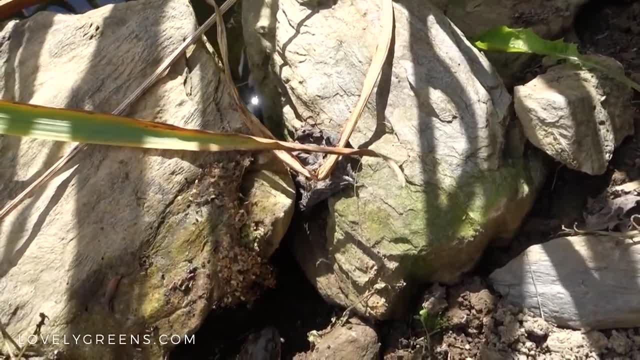 intention, as well as to create a haven, a place for insects and birds to come in place, for insects and birds to come in place, for insects and birds to come in and have a drink and also to try to and have a drink and also to try to. 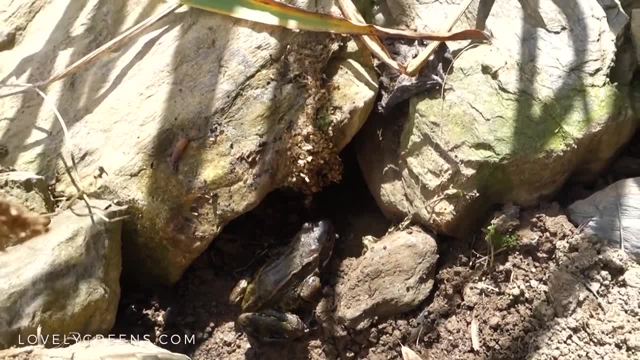 and have a drink and also to try to attract frogs, and I was successful last attract frogs and I was successful last attract frogs and I was successful last year in attracting a frog and I had some year in attracting a frog and I had some year in attracting a frog and I had some tadpoles in my pond as well and frogs. 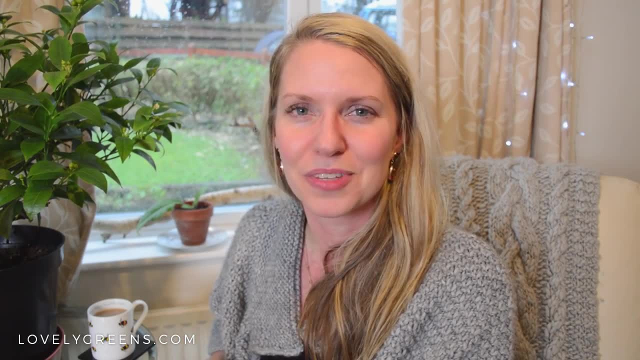 tadpoles in my pond as well, and frogs tadpoles in my pond as well, and frogs are excellent eaters of slugs, so I'm are excellent eaters of slugs, so I'm are excellent eaters of slugs, so I'm hoping that even more frogs make my my. 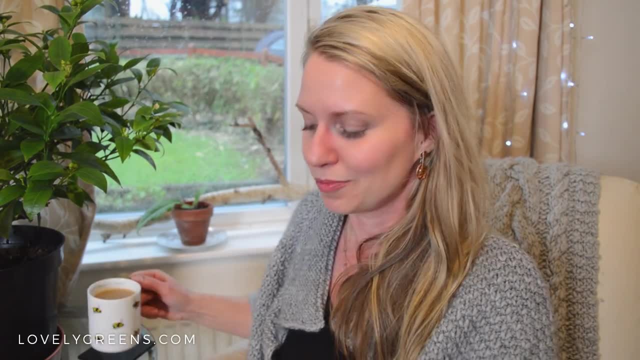 hoping that even more frogs make my my. hoping that even more frogs make my my. small garden pond their home this year. small garden pond their home this year. small garden pond their home this year. fingers crossed because here in Britain, fingers crossed because here in Britain, fingers crossed because here in Britain, Isle of Man, so many slugs, it is the. 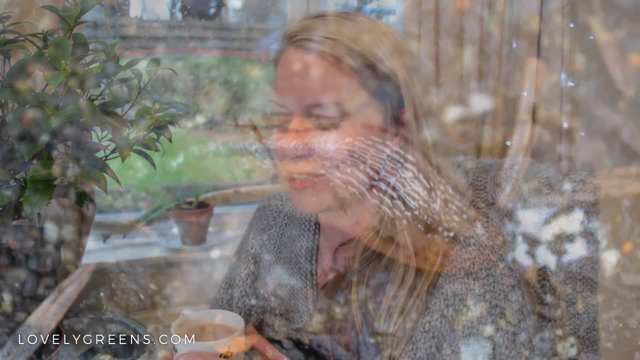 Isle of Man, so many slugs. it is the Isle of Man- so many slugs. it is the number one pest in my allotment garden. number one pest in my allotment garden, number one pest in my allotment garden other than the New Zealand flatworms of 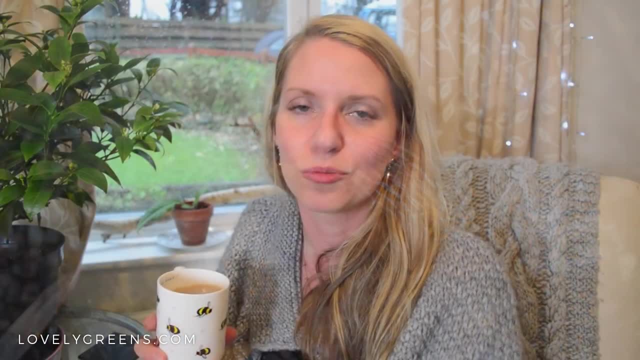 other than the New Zealand flatworms, of other than the New Zealand flatworms, of course, course, course. another thing that I did recently was another thing that I did recently was another thing that I did recently was put in some supports for my my, put in some supports for my, my. 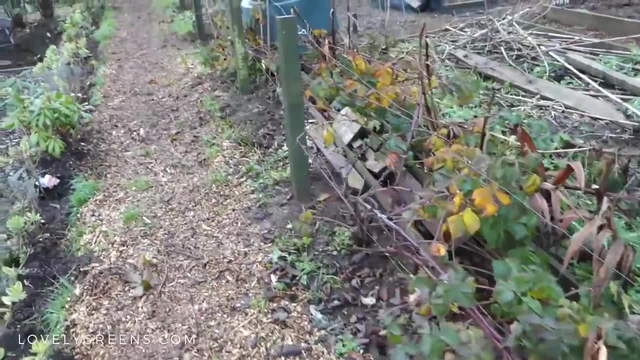 put in some supports for my my thornless blackberries and projects like thornless blackberries and projects like thornless blackberries and projects like this are great this time of the year. I this are great this time of the year. I this are great this time of the year. I mean it's rainy outside, but it isn't it. 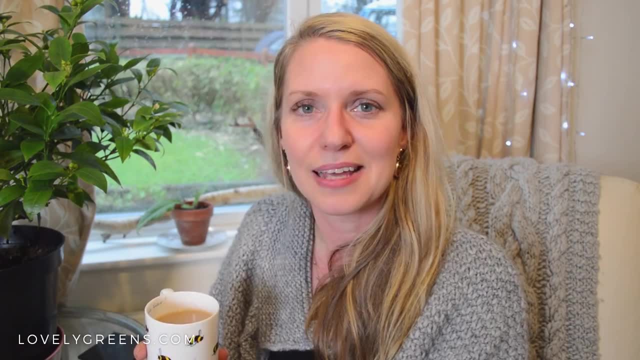 mean it's rainy outside but it isn't. it mean it's rainy outside but it isn't. it isn't too cold or snowy. and if you have isn't too cold or snowy, and if you have isn't too cold or snowy, and if you have kind of the same climate or it's a. kind of the same climate. or it's a kind of the same climate or it's a little bit further into the winter, for little bit further into the winter, for little bit further into the winter for you and you're looking for some things, you and you're looking for some things. 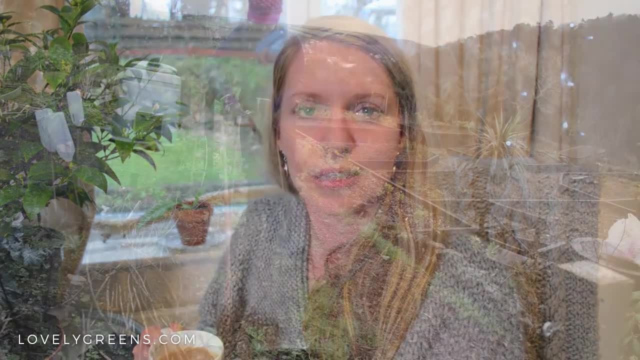 you and you're looking for some things to do: putting in kind of permanent to do. putting in kind of permanent to do, putting in kind of permanent features like supports and pathways and features like supports and pathways, and features like supports and pathways and edging and things like that. this is what 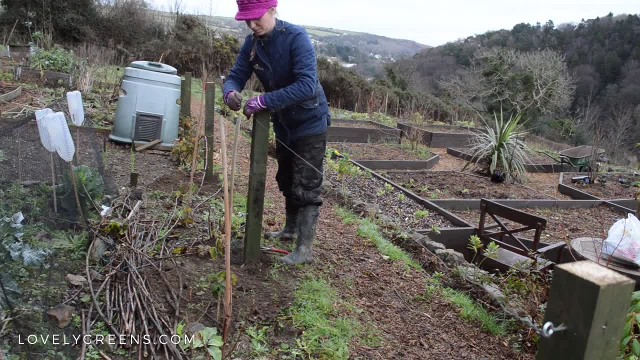 edging and things like that. this is what edging and things like that. this is what you can do to prepare for spring. because you can do to prepare for spring, because you can do to prepare for spring, because you know when spring starts rolling. you know when spring starts rolling. 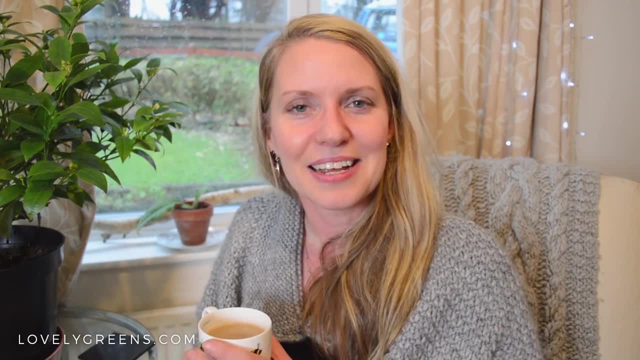 you know, when spring starts rolling around, you're not gonna have time to do around, you're not gonna have time to do around, you're not gonna have time to do it. so, in any case, I wanted to share a it. so, in any case, I wanted to share a.